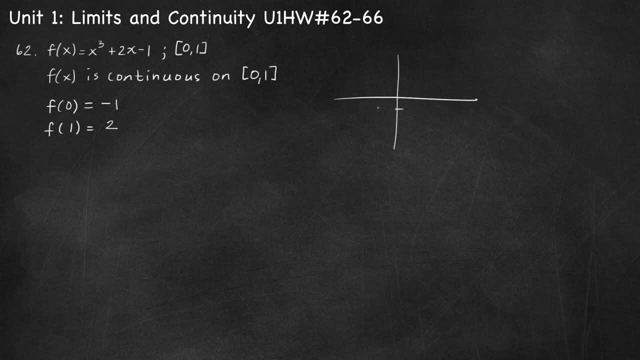 about our function. We know that f of 0 is negative 1 and the f of 1 is 2. And we know that our function is continuous. So I'm not sure exactly what this looks like here. although I could graph, I do have my equation so I could. 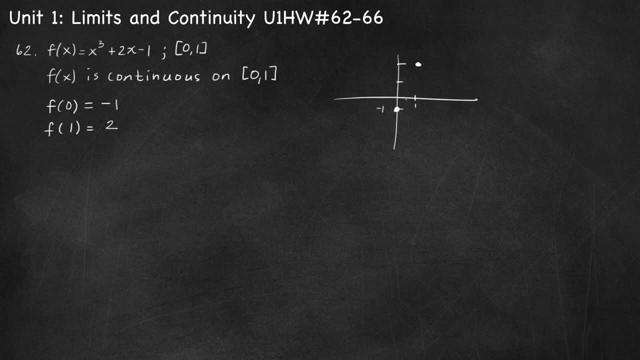 graph it and get a better idea of exactly what this looks like. But since it's continuous, I know that I have to get somehow. I have to get from this first endpoint up to the other endpoint. Now it doesn't have to look exactly the way I drew it, but somehow with a smooth 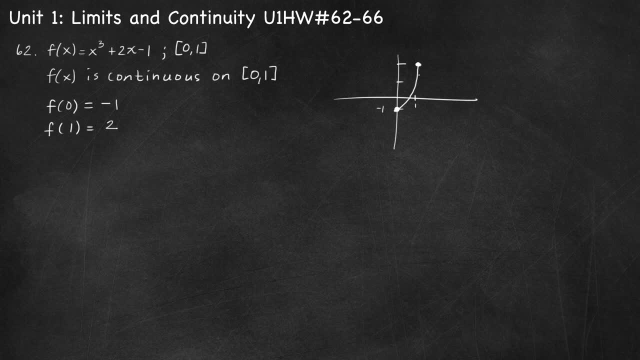 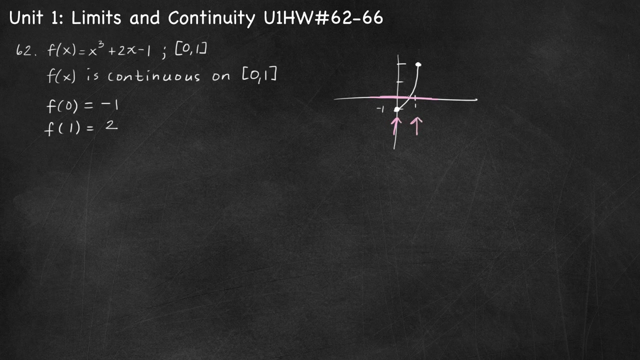 continuous curve. I have to get from that one point to the other point, And so, yes, there must be a place where my function is equal to 0. There has to be a place between and, furthermore, we know where it is: it's somewhere between 0 and 1.. That has to occur. Okay, so, since f is continuous, on. 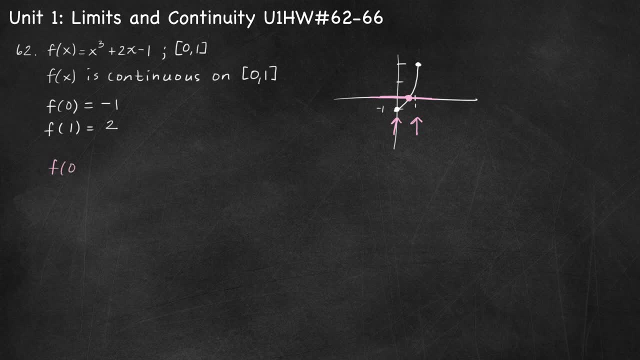 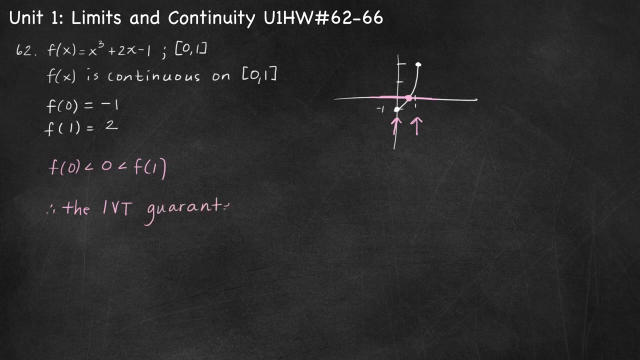 the interval from 0 to 1 and 0 is in between f of 0 and f of 1. So I have to get somewhere between 0 and 1.. Therefore, the IVT, or intermediate value theorem, guarantees that there exists some value. 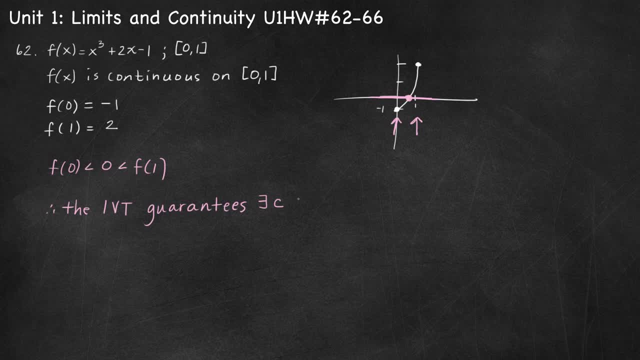 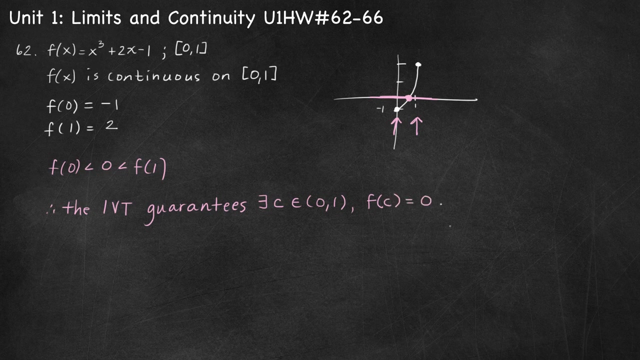 c. Now c is an x-coordinate. so there exists some x-coordinate c on the open interval from 0 to 1, such that our function at that x-coordinate f of c is equal to 0. So I have to get somewhere between 0 and 1 and f of c is equal to 0. Okay, so again, c is an x-value, f of c is the corresponding y-value. 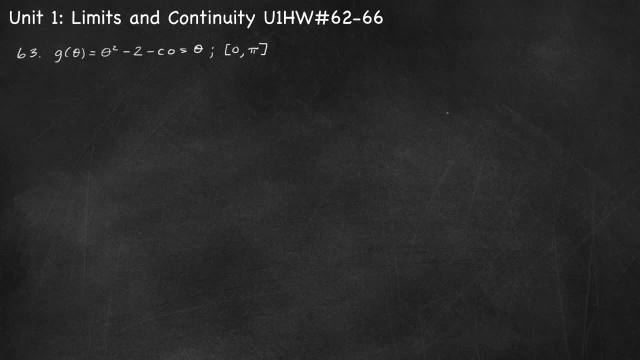 63.. Show, using the intermediate value theorem, whether or not the function g of theta equals theta squared minus 2 minus cosine. theta has a 0 on the interval from 0 to pi. Well, our function needs to be continuous in order for us to use the intermediate value theorem. 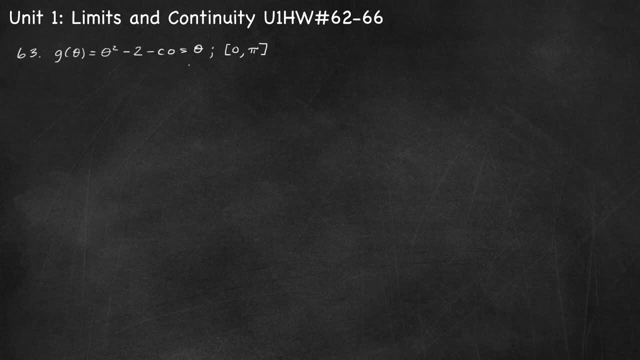 If we look at the interval from 0 to pi, we'll see that the function g of theta equals theta squared, and that term is continuous. So again now we have to suggest that each term here, each term is continuous. theta squared is continuous. negative 2 is continuous. Negative cosine: theta is continuous. 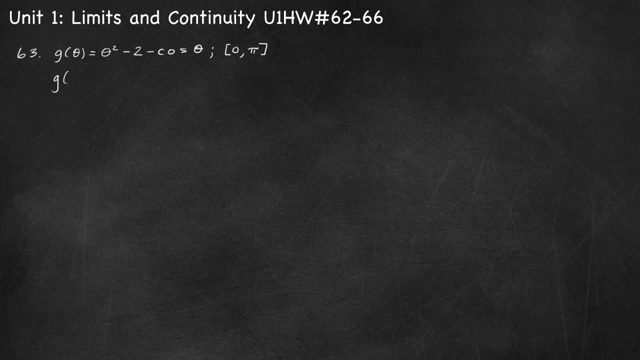 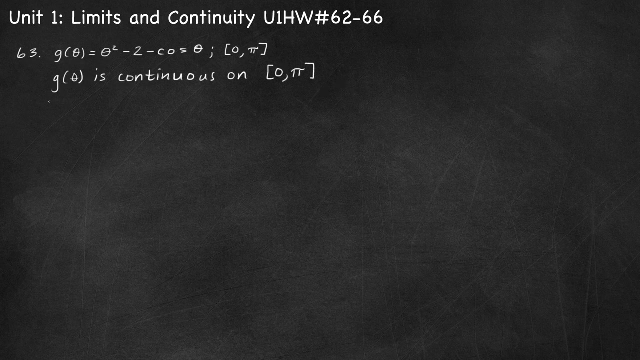 And the sum of continuous functions is continuous. So we do have g of theta is continuous. it's actually continuous for all real numbers, but we only need it to be continuous on the closed interval from 0 to pi. So g of theta is continuous on the interval from 0 to pi. Now let's check our endpoints. g of 0 and then g of j. So g of j is continuous. Now let's say I've got some of these values. So g of 0 and then g of j of 1 is continuous. So g of theta has � Anyways let's put this in the next section here where g of 0 is continuous. 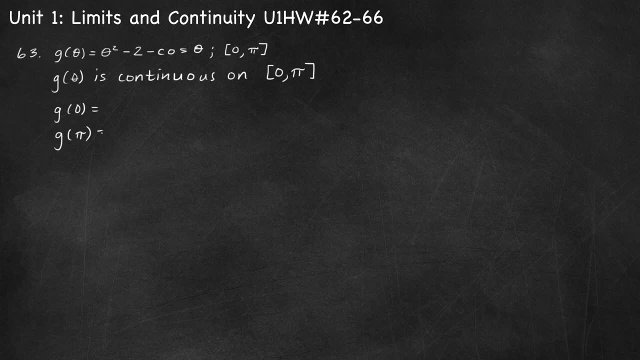 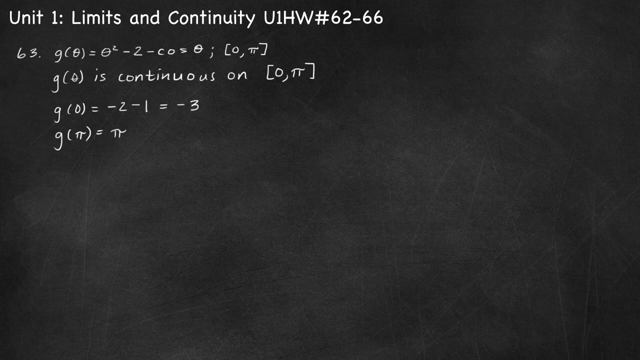 So we know that we have a continuous interval interval. And if we come back here and wanted to get rid of a small interval period, zero and then g of pi. so at g of zero we have zero squared minus two minus the cosine of zero. the cosine of zero is one, so g of zero is negative three. for g of pi, we have pi squared minus two. 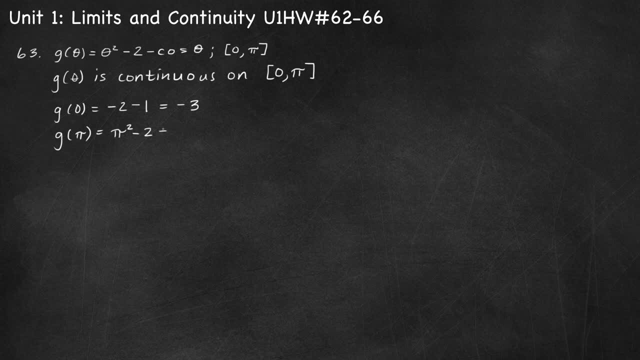 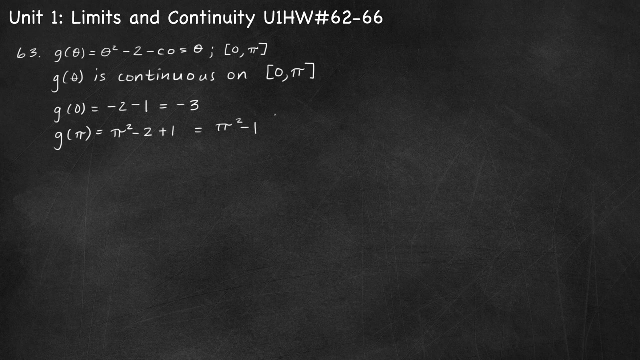 minus the cosine of pi. and the cosine of pi is negative one, so we're subtracting negative one- and that will simplify- to pi squared minus one. we want to know if g has a zero between zero and pi. so that's somewhere the equation is equal to zero, so our y-coordinate in question is zero and that. 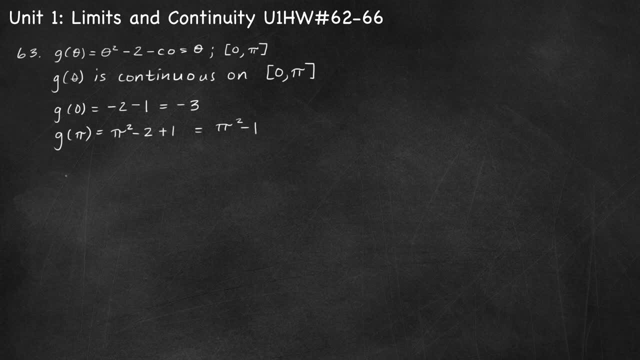 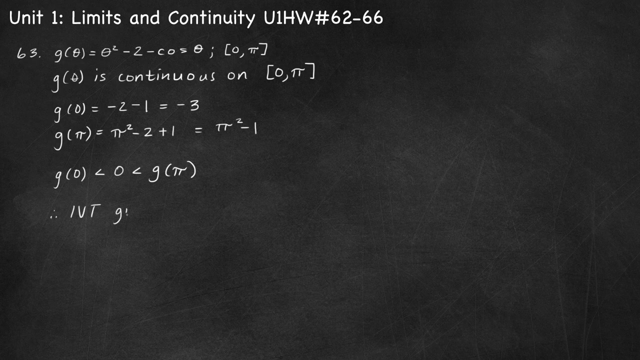 is in fact between negative three and pi squared minus one. so negative three is less than zero, which is less than pi squared minus one. therefore the intermediate equation is equal to zero, and that is equal to pi squared minus one. so the intermediate value theorem does guarantee that there exists some value c, some x value c on the interval from zero to pi. 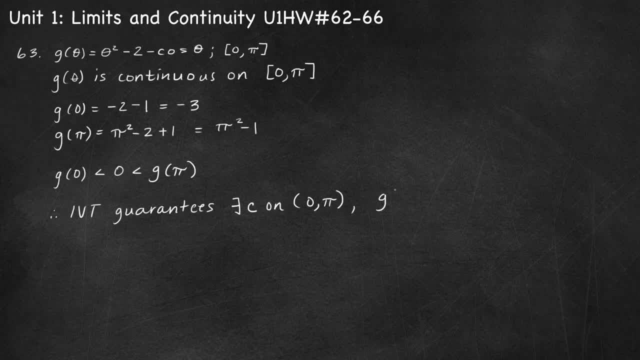 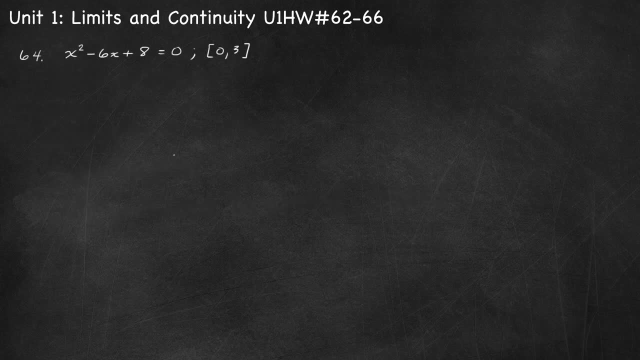 such that our function, evaluated at c, will equal zero 64. determine whether the IVT can be used to show that x squared minus 6x plus 8 equals zero on the interval from zero to three. if so, find the value of c guaranteed by the theorem. 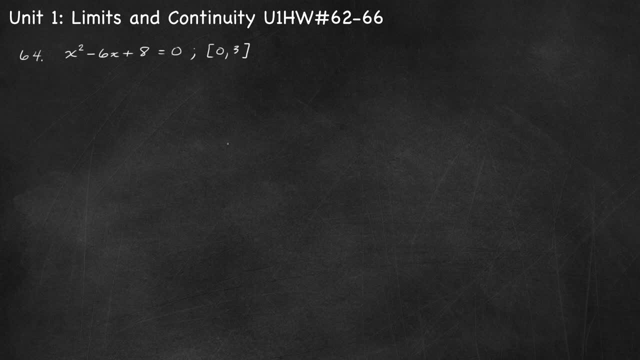 x squared minus 6x plus eight is a polynomial function. so we know that it is continuous for all real numbers. so it certainly is continuous between 0 & 3. so our function, we i could call it f of x if i wanted to. i'll just 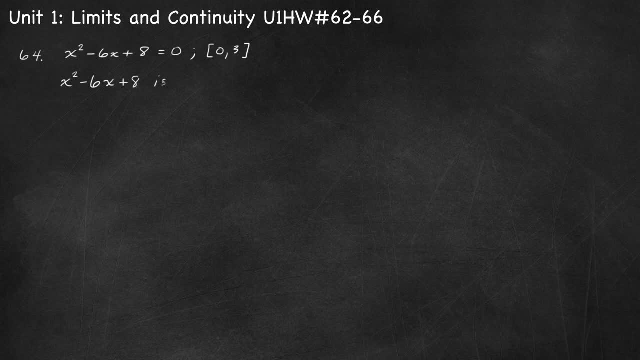 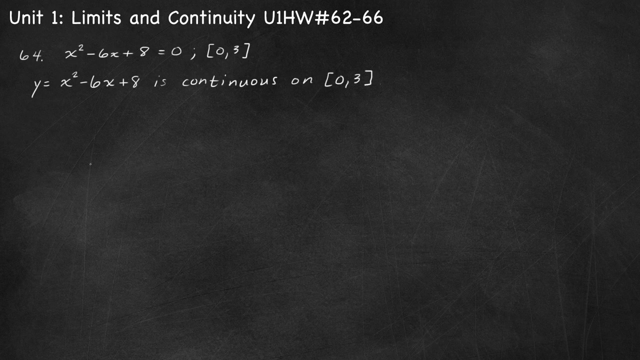 say x squared minus 6x plus 8 is continuous. I guess we should call it something. Let's just say that x cubed minus 6x plus 8 illegal- say y equals is continuous on that interval from zero to three. Now let's consider our y. 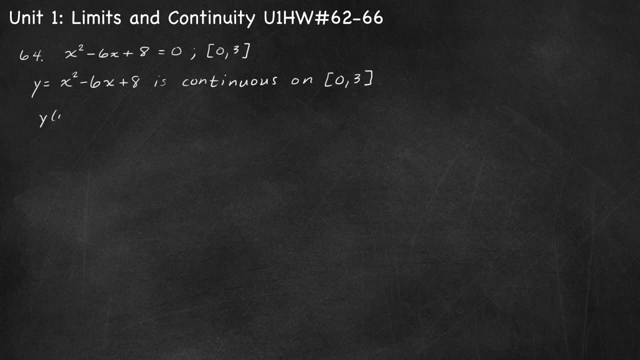 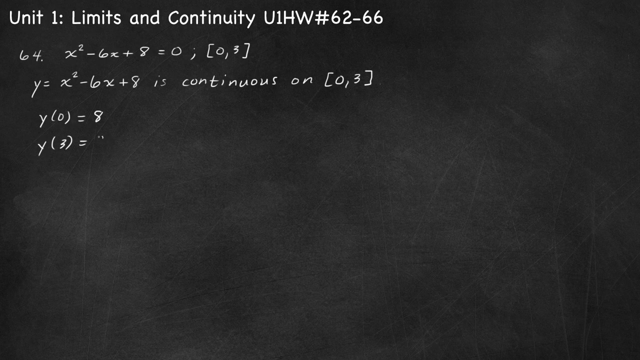 coordinates at our endpoints. So we have now y of zero and then y of three. At zero our function becomes zero squared minus six times zero plus eight, or just eight At three we get three. squared, it's nine minus six times three, so minus eighteen plus eight, or negative one. And we want to know is: 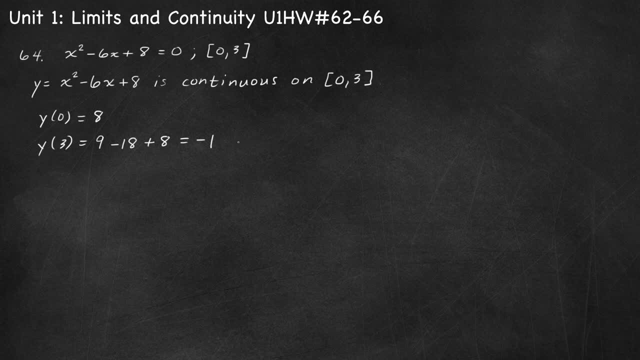 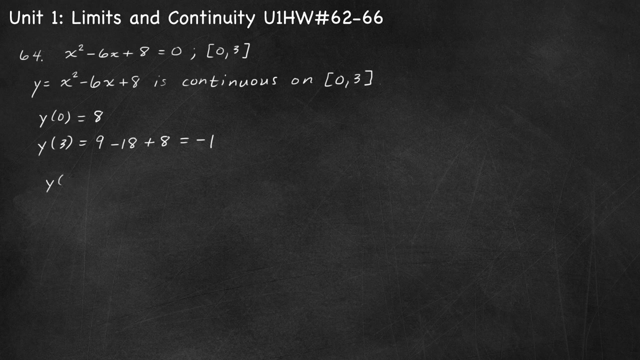 there somewhere the equation is equal to zero. That zero is our y coordinate. Is that y coordinate in between eight and negative one? Yes, it is. This time our left endpoint is higher than zero and our right endpoint is lower than zero. That's okay, we still have it being in between. 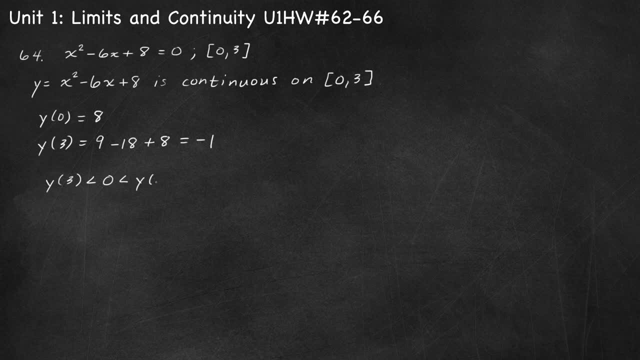 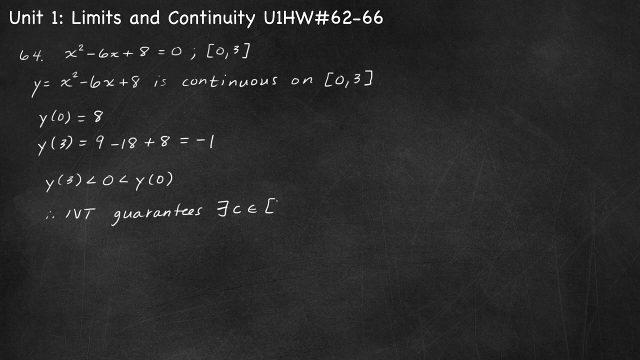 So zero is in between y and eight, y of 3 and y of 0. Therefore the IVT does guarantee the existence of a value c in the interval between 0 and 3, and that should be open interval 0 to 3,. 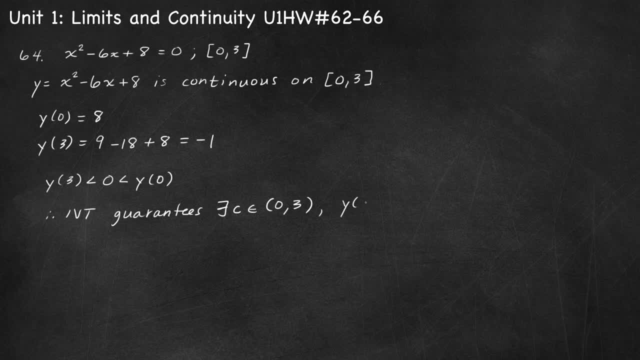 such that our function y at that value c is equal to 0. And in this problem we were asked to go a step further and find that value of c. So to do that, we just set our equation equal to 0 and solve it, and we know our solution. 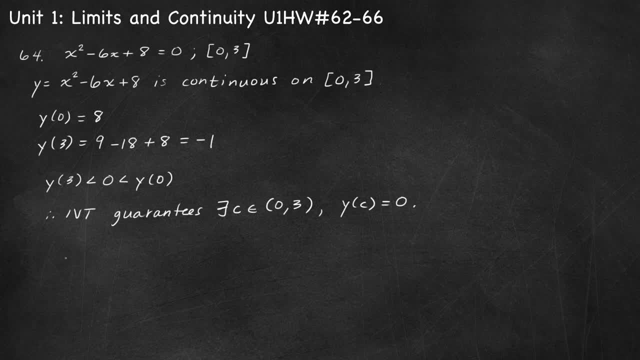 will be some x value between 0 and 3.. So x squared minus 6x plus 8 equals 0. Let's see if that's factorable. That's probably the quickest way to go. So minus 2, minus 4.. 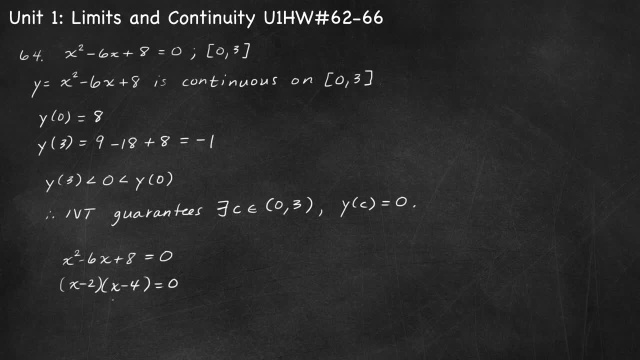 Let me quickly multiply that back out, make sure it's right. So x squared minus 6x plus 8 equals 0.. x squared minus 6x plus 8, yes, So we have x equals 2 and x equals 4. 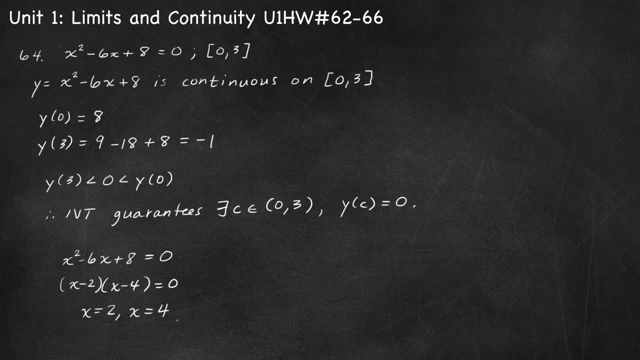 as solutions for this equation. However, the intermediate value theorem only guarantees a c between 0 and 3.. It does not guarantee the 4.. Now, x equals 4 is a solution, It is a 0,, but it is not one that is guaranteed. 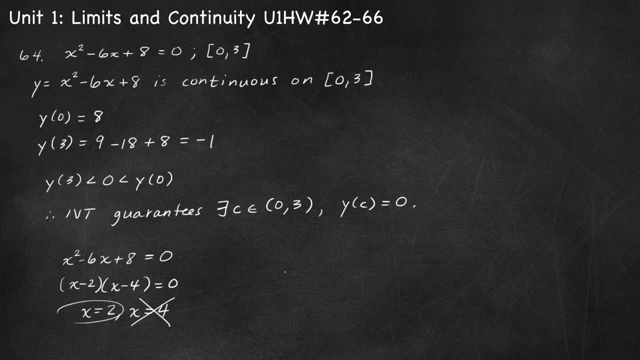 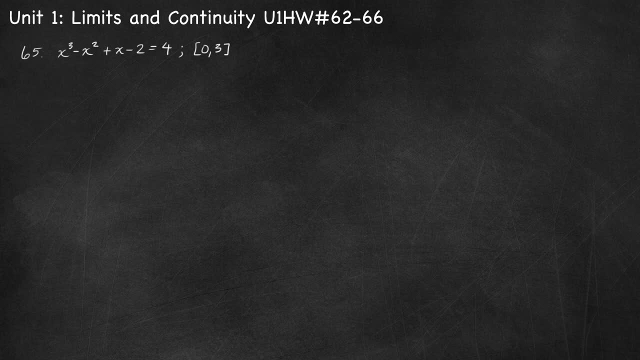 by the intermediate value theorem. So the value of c we're looking for is just the 2.. Number 65. Determine whether the IBT can be used to show that x cubed minus x squared plus x minus 2 equals 4 on the interval from 0 to 3.. 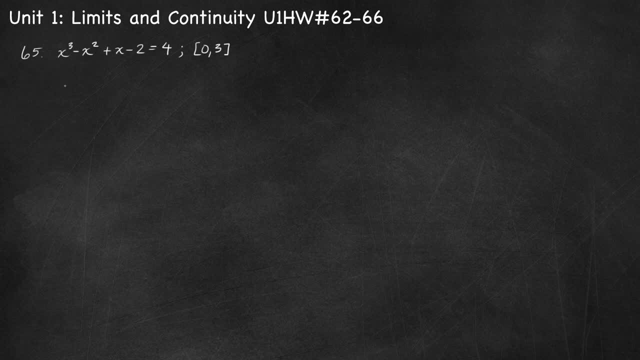 If so, find the value of c guaranteed by the theorem. Our function on the left-hand side here is a polynomial, so it is definitely continuous on the interval from 0 to 3.. And I'm just going to call that left-hand side f of x. 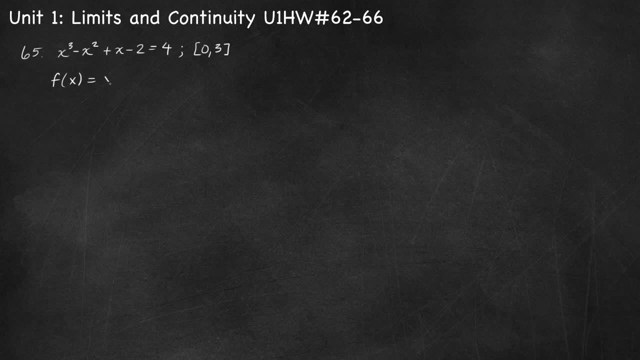 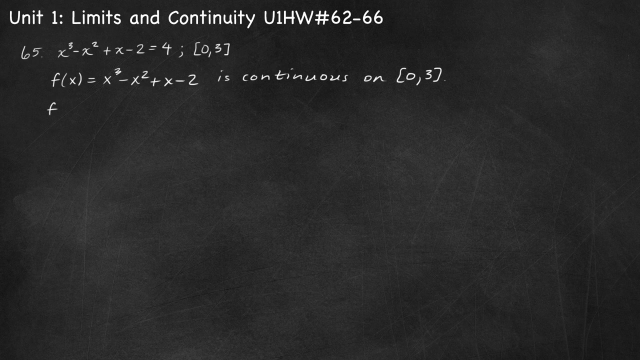 to help me with my notation here. So f of x equals x cubed minus x. x squared plus x minus 2 is continuous on that closed interval from 0 to 3.. And let's find our endpoints: f of 0 and then f of 3.. 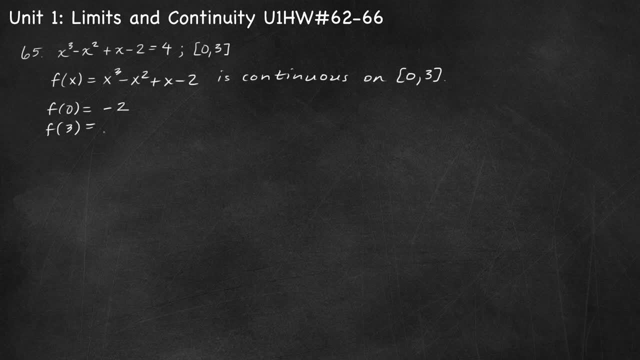 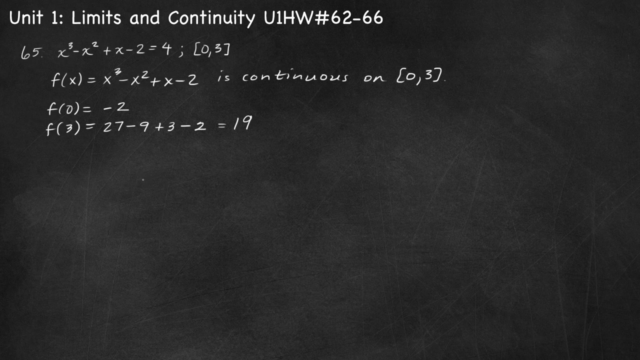 So f of 0 is negative. 2. f of 3. So we've got 3 cubed minus 3 squared plus 3 minus 2. So f of 3 is 19. And we are looking to see. is there somewhere this equation? 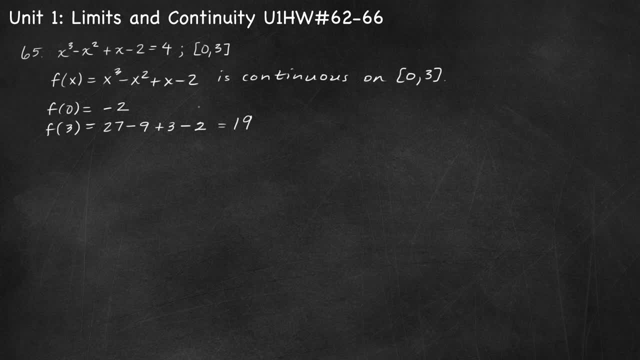 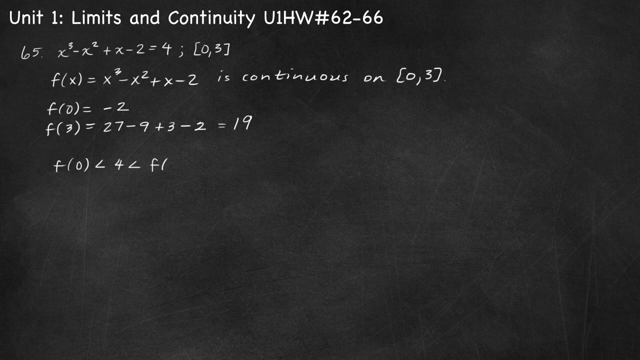 equals 4.. So the y coordinate of 4 is between these two y coordinates, at the endpoints negative 2 and 19.. So the IBT does apply in this case. So we can say: f of 0 is less than 4, which is less than f of 3.. 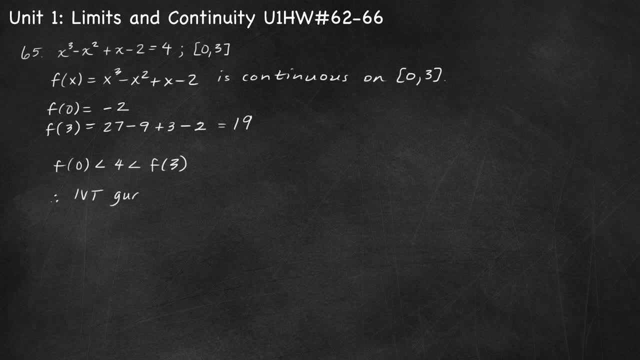 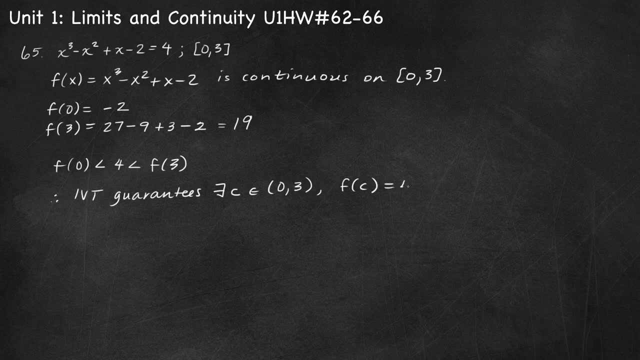 Therefore The Intermediate Value Theorem guarantees that there exists a value c on the interval open interval from 0 to 3, such that f of c is equal to 4.. Now we're asked to find that value. So we're going to let x cubed minus x squared plus x minus 2. 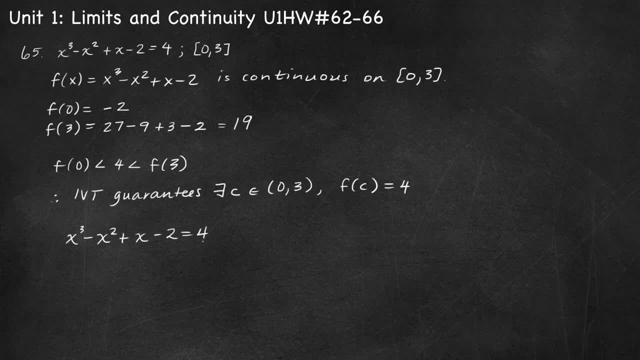 equal 4 and solve And we can subtract 4 on both sides: x cubed minus x squared plus x minus 6 equals 0.. So it doesn't look like I can factor this by grouping. I'd probably just try a guess and check at this point. 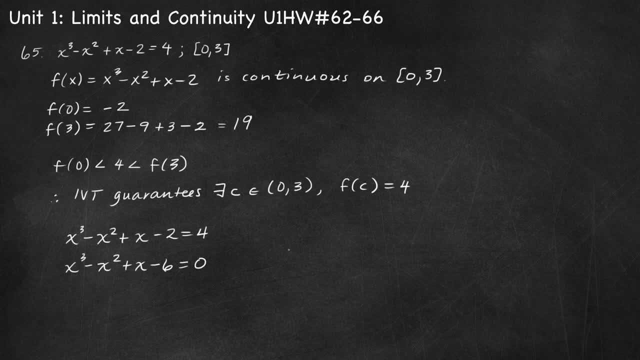 Or if we can use our calculator, we can graph and find a solution. that way, If I'm doing guess and check, I'm going to try easy values like 1 or negative 1, 2, negative 2, 0.. 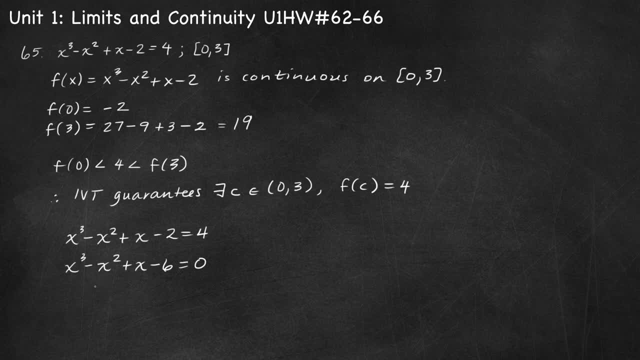 And just doing a quick guess and check, it, looks like 2 is going to work. That 2 is going to give me 8 minus 4 plus 2 minus 6, which is going to be 0. So I have x equals 2, and that is indeed on our interval from 0 to 3.. 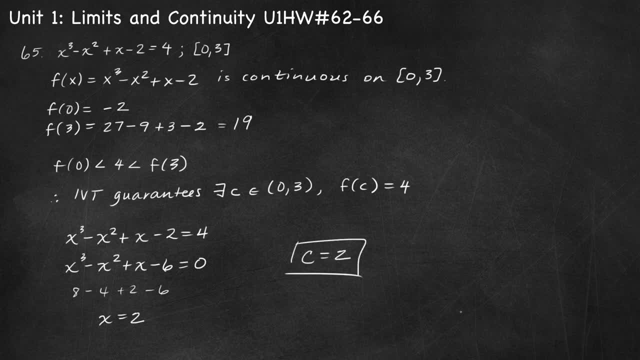 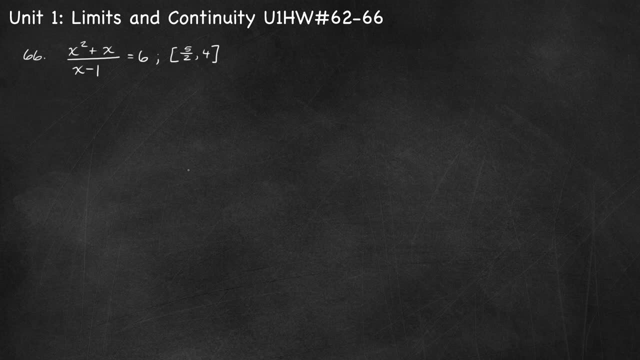 So the c value is 2 and 66.. Determine whether the IVT can be used to show x squared plus x over. x minus 1 equals 6 on the interval from 5 halves to 4.. If so, find the value of c guaranteed by the theorem. 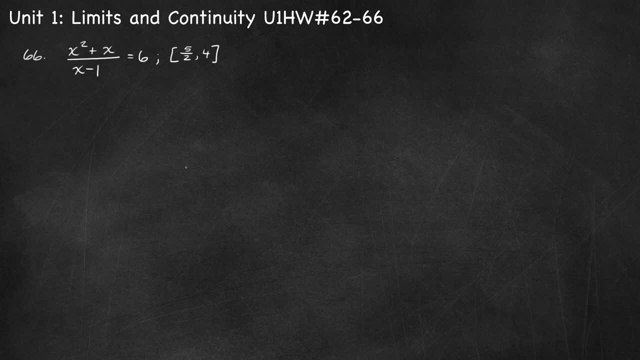 Now, this is not a polynomial function. It is not continuous. for all real numbers, I can see that there is a discontinuity at x equals 1.. However, 1 is not in my interval, And if it's outside the interval it's okay that there's a discontinuity there. 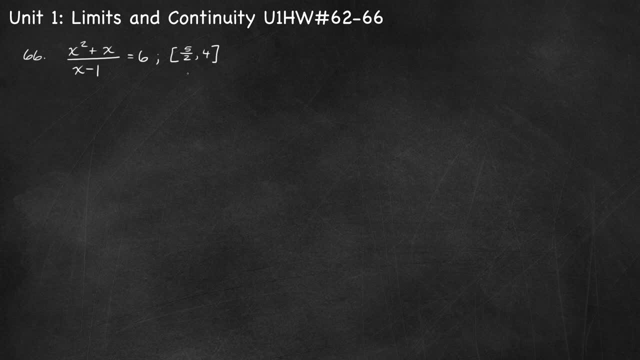 I just need the graph to be continuous. It's from 5 over 2 to 4, or 2.5 to 4.. So let's call the left-hand side f of x again. So I can say: f of x equals x squared plus. x over x minus 1 is continuous. 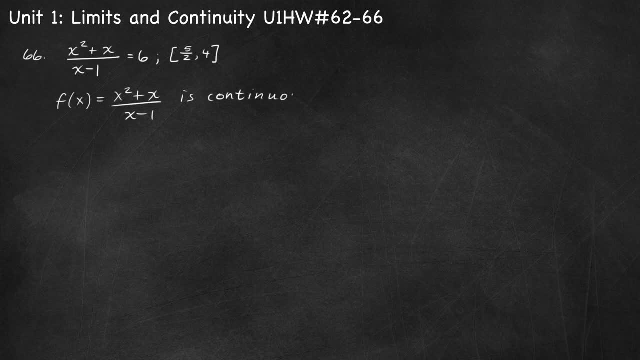 Let's spell that correctly- Is continuous on the closed interval from 5 over 2 to 4.. And I know that it's continuous there because I can see from the equation that it's continuous. It's continuous everywhere except for x equals 1.. 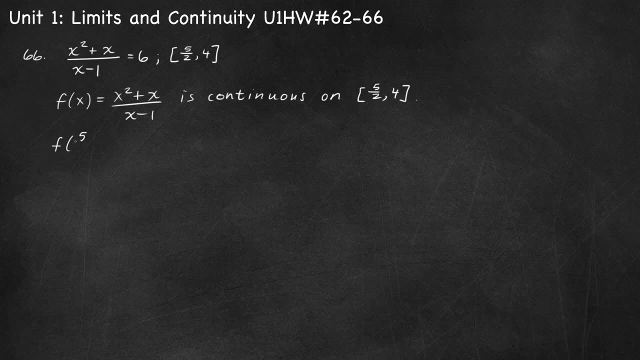 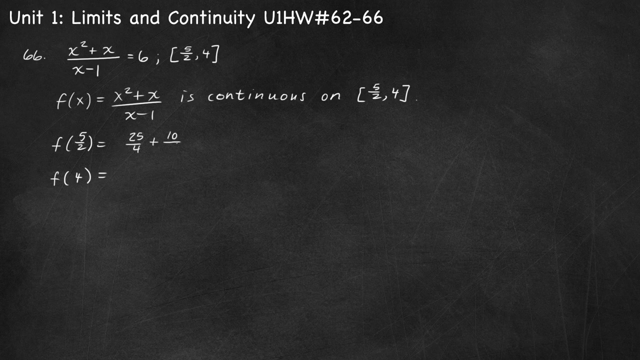 Let's check our endpoints. So f of 5 over 2, and then we need f of 4.. So 5 over 2 squared is 25 over 4 plus 5 over 2,. if I want a common denominator, let's go with 10 over 4,. 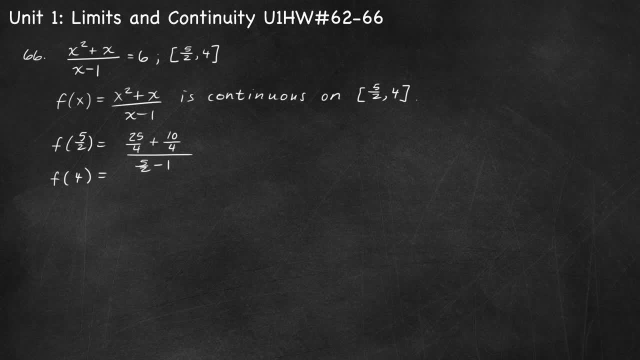 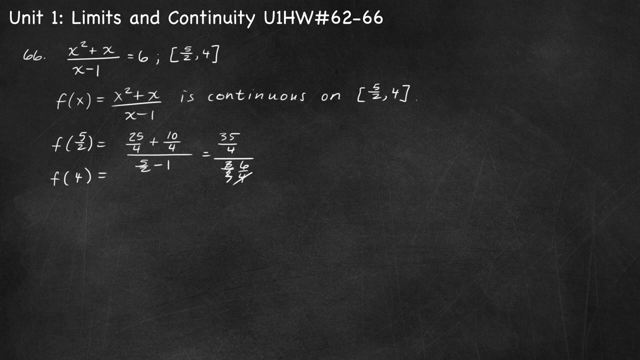 over 5 over 2 minus 1.. So that's 35 over 4, over 5 over 2 minus 2 over 2 is 3 over 2.. If I make that 6 over 4, then I can just cancel out my denominators. 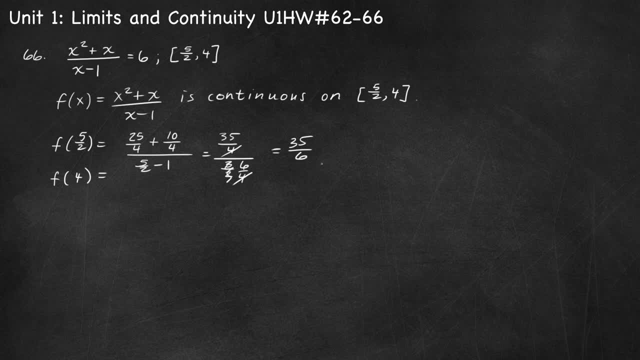 This is 35 over 6, or a little bit less than 6.. Now f of 4, let's move that down a little bit. f of 4, I'd have 4 squared plus 4 over 4 minus 1.. 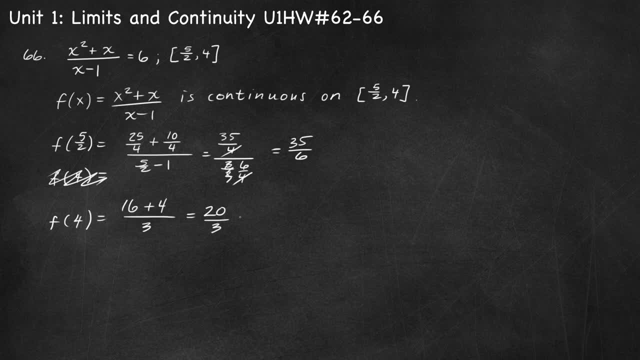 So 20 over 3, and 20 over 3 is going to be a little bit more than 6.. So 35 divided by 6 is a little bit less than 6, and 20 divided by 3 is a little bit more than 6.. 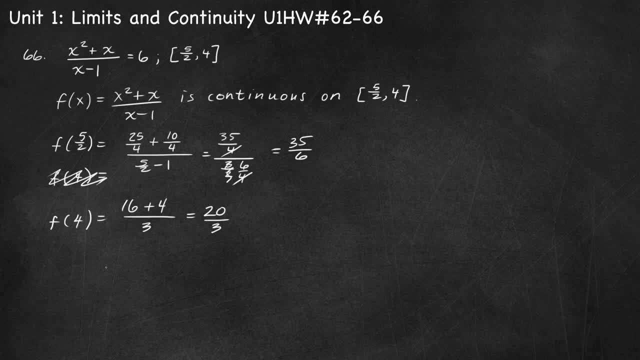 So thankfully, the number we're looking for- 6, is in between those values. So f of 5 over 2 is less than 6,, which is less than f of 4.. Therefore the intermediate value theorem guarantees that there exists a value c on our interval from 5 over 2 to 4,. 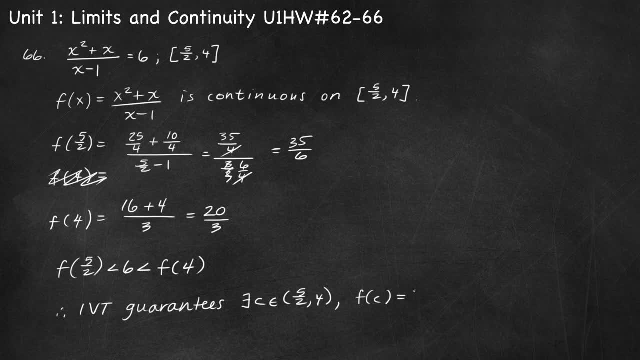 such that f of c equals 6.. Now we're asked to find that value. so we're going to solve our equation: f x squared plus x over x minus 1, equals 6.. So I'm going to subtract the 6 to get the right hand side equal to 0.. 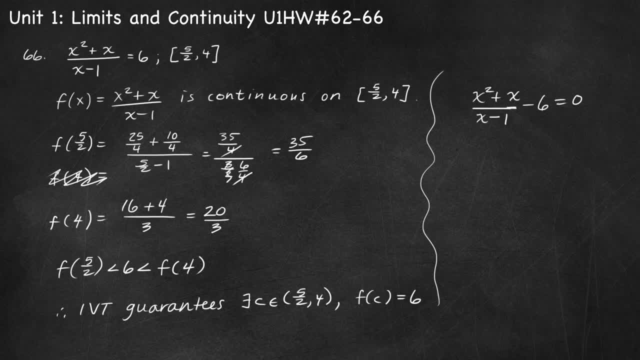 And now let's make this all one fraction. So x squared plus x minus 6 times x minus 1, over x minus 1, equals 0.. And the only time a fraction will equal 0 is when its numerator is 0.. 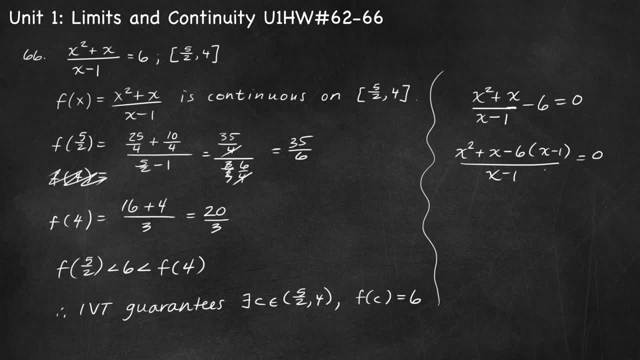 So for now I can just ignore that denominator and I just want to know when does this numerator equal 0.. So let's simplify the numerator. We get x squared plus x. minus 6x is going to give me negative 5x. 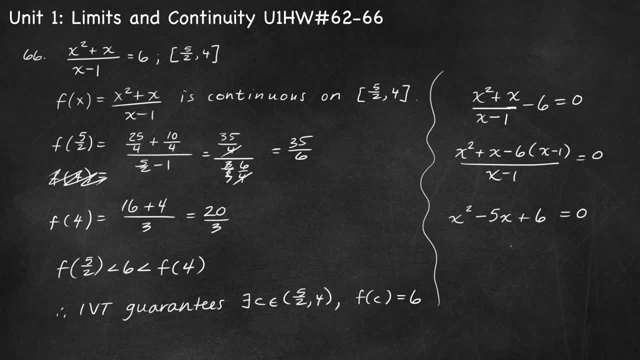 and then plus 6 when I distribute that And this looks like it is factorable. So x minus 6 and positive 1. Let's see x squared minus 5x minus 6.. Nope, that does not work. Let's try 2 and 3..